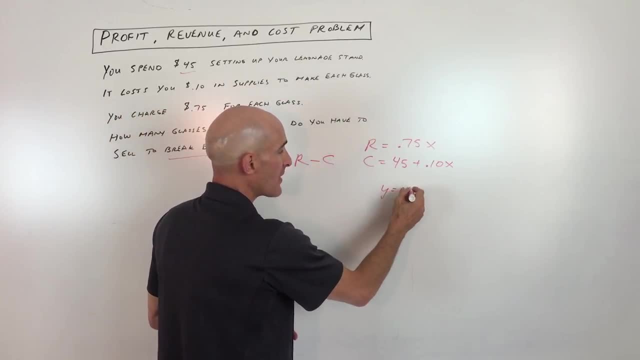 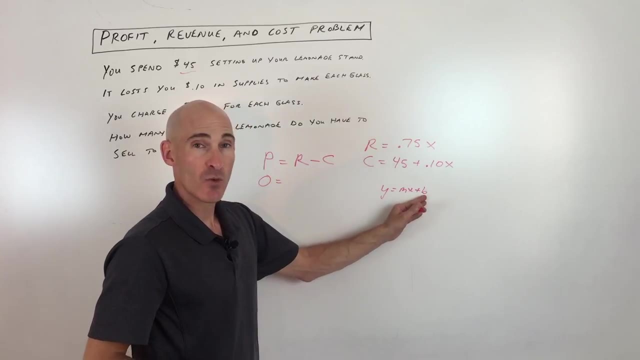 about these two equations is if you think about the y equals mx plus b form of the line, you probably learned the slope intercept form of the line. The m is the slope and the b is the y intercept. but when you're doing word problems such as these, the slope is really the rate okay. 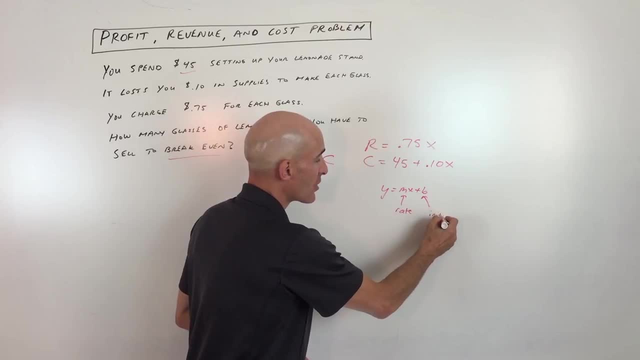 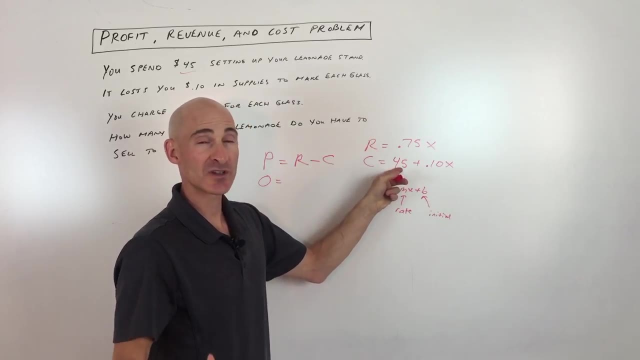 and the b, the y intercept is really the initial or the starting amount. okay, the initial condition. So in this case, the initial condition here is the $45 that you spent, that one-time fee to get your lemonade stand up and running, and then the rate is the 10 cents that it costs you each glass that. 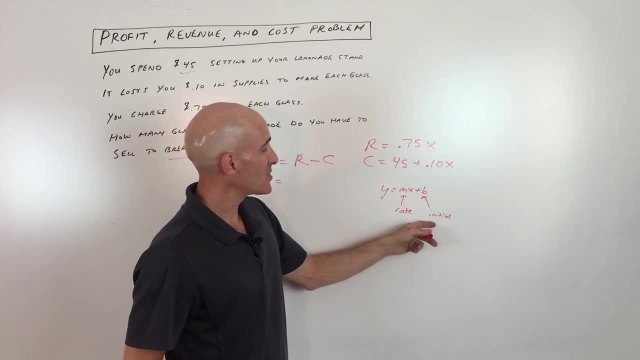 you make Over here with the revenue. there's no initial quantity for the revenue. it's not like you're getting a one-time lump sum. you're just getting a 75 cents per each glass. so that's the rate, okay, that you're getting. So that's the rate, okay that you're getting. So that's the. 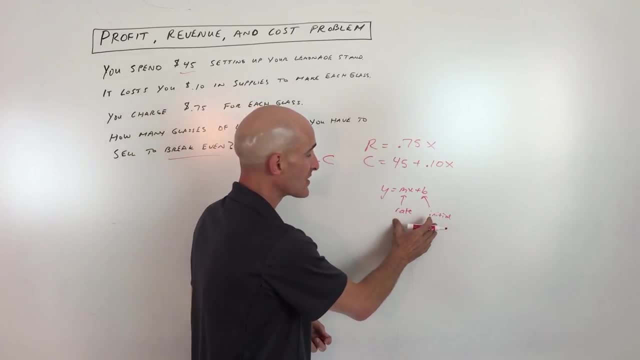 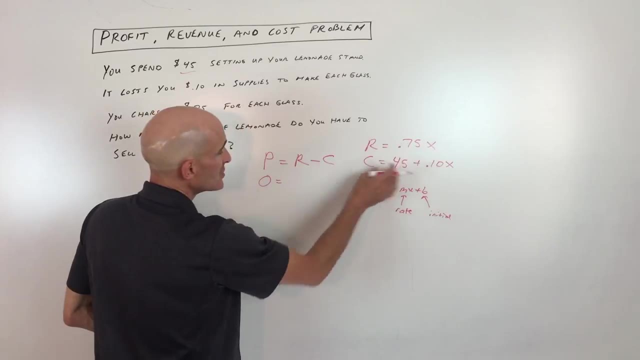 per each glass. So that helps a little bit. when you're doing word problems like this, Think about not the slope but the rate, and then not the y intercept but the starting amount or the initial amount. So then all we have to do is substitute these quantities into our equation. The revenue: 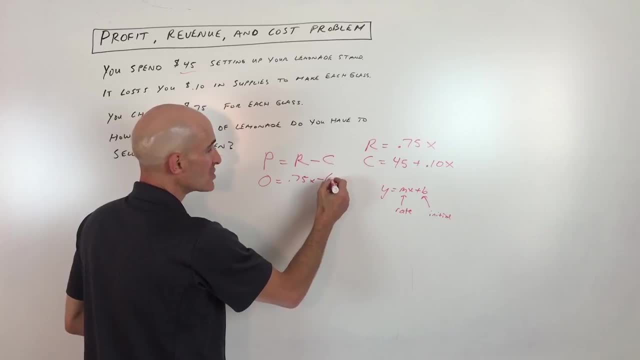 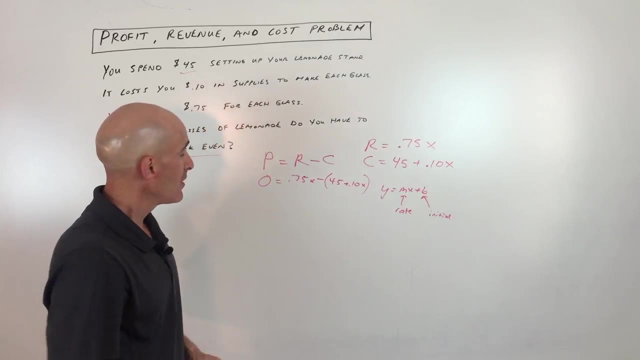 is 0.75x minus the cost, which is 45 plus 0.10x. Notice I put it in the parentheses because we want to subtract that whole quantity. So now what we're going to do is we're going to solve for x. 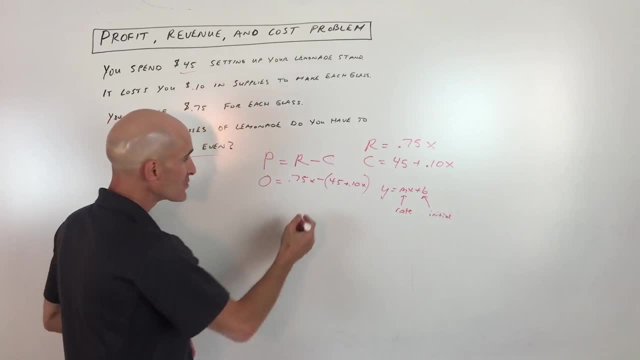 the number of glasses to reach that break-even point. So let's go ahead and distribute the revenue here, So that gives us 0.75x minus 45 minus 0.10x combined like terms, right, So that's. 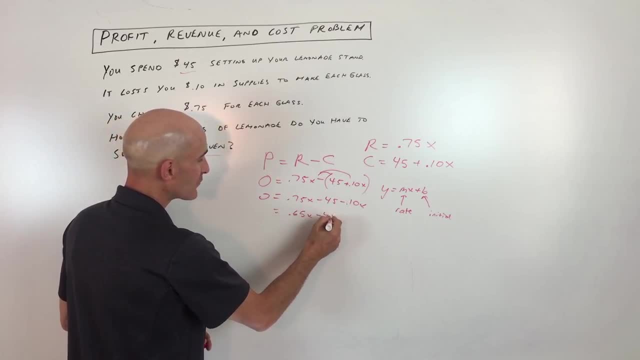 going to give us 0.65x minus 45 equals 0.. We're going to add the 45 over here: equals 0.65x, and then we're going to divide both sides by 0.65 to get x by itself. So I'm going to go to the 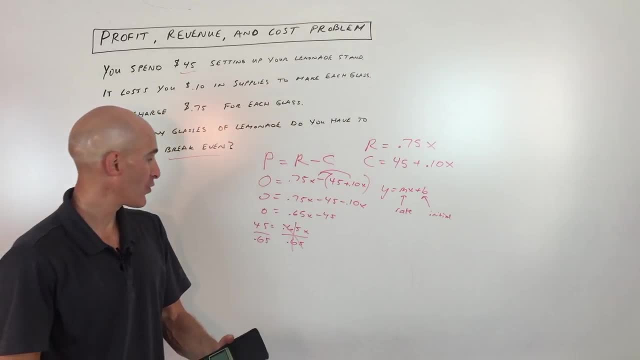 calculator now: 45 divided by 0.65.. 45 divided by 0.65, we get 0.65x minus 0.10x, So that's going to be 69.2.. Okay, now here's the thing. Can you sell 0.2 glasses of lemonade? Probably not, So. 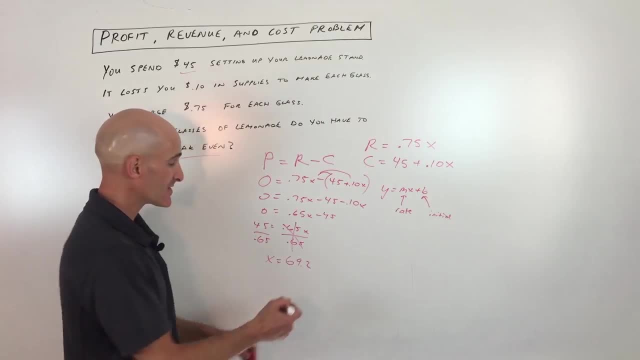 really to reach that break-even point. we're going to just round this up to 70 glasses- approximately 70 glasses of lemonade- until you reach your break-even point. After that you're going to become profitable when you sell that 71st glass, 72nd glass, etc. Normally those 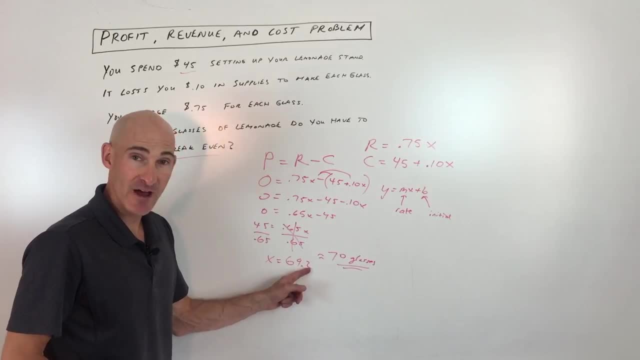 students would think to themselves: hmm, this is 0.2, that's less than 5,. right, I would round down that. But in this case, if you only sell 69 glasses of lemonade, you actually haven't recouped. 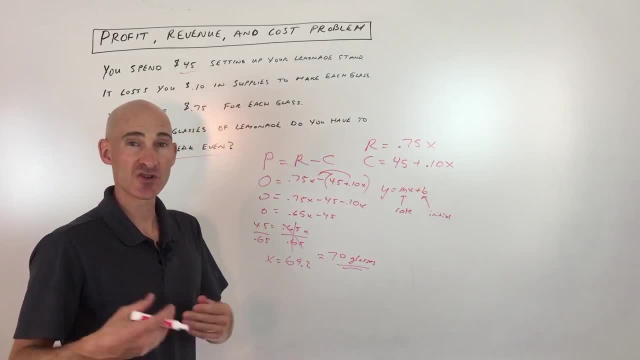 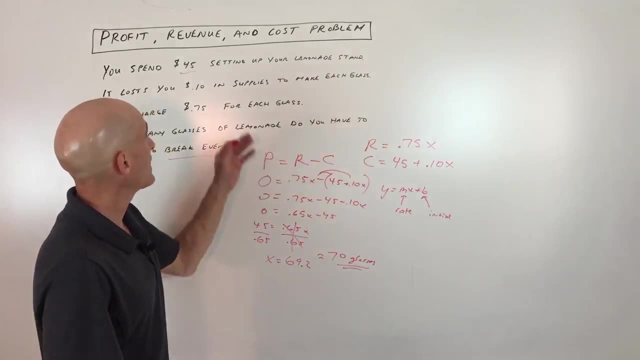 that initial cost for the $45 that you had to spend to get your lemonade stand up and running. So it's going to take that 70th glass to basically break even and then go into profitability. So again, I hope this helps you understand how to work with these types of word problems. Again, 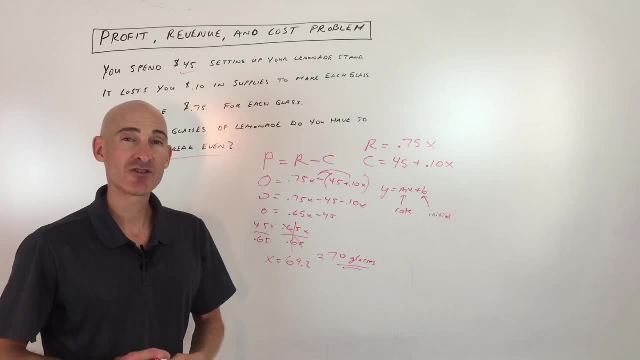 think about some of the tips that we talked about here. Subscribe to the channel. Check out some of my other videos on Mario's Math Tutoring YouTube channel and I look forward to helping you in the future videos. I'll talk to you soon. 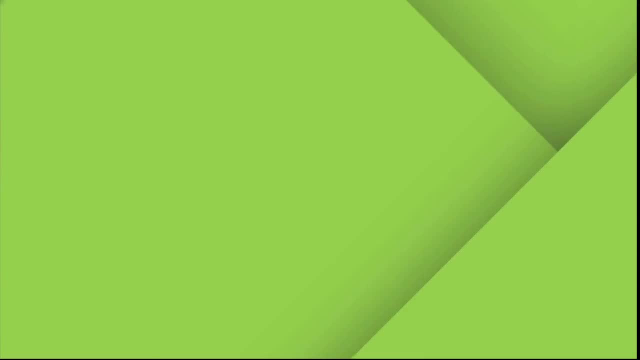 So how are the areas of a rectangle and triangle with the same base and height related? I'm Bon Crowder with Math4.com, coming to you from Terry Pro Graphics in beautiful Houston, Texas. Here we have a rectangle with a base and a height and a triangle with the same base and height. 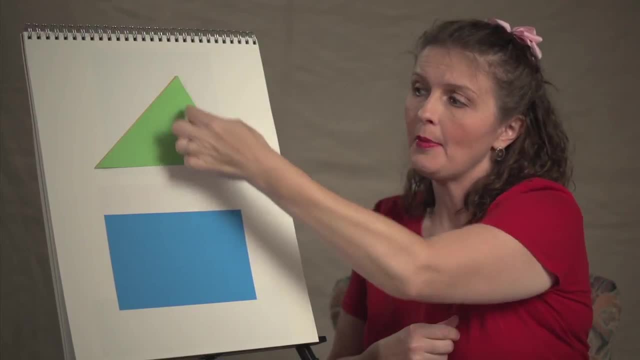 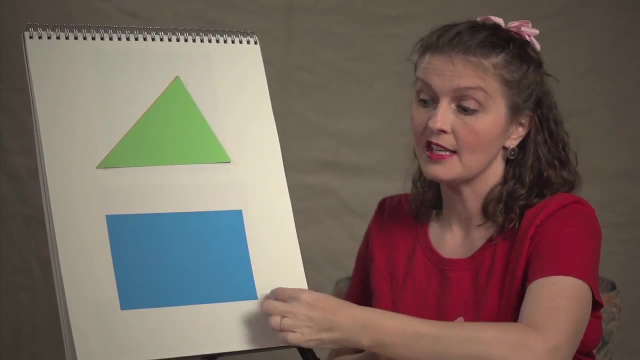 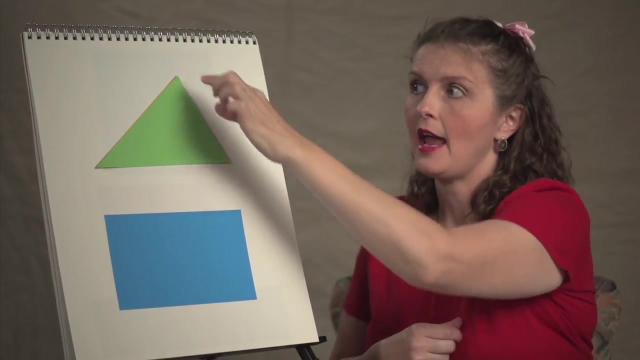 Remember, the height of a triangle is from the tip perpendicular to the base. That's the same on a rectangle, but it's also the edge, because it is perpendicular to the base. So let's look at this triangle a little differently than the way it is now. 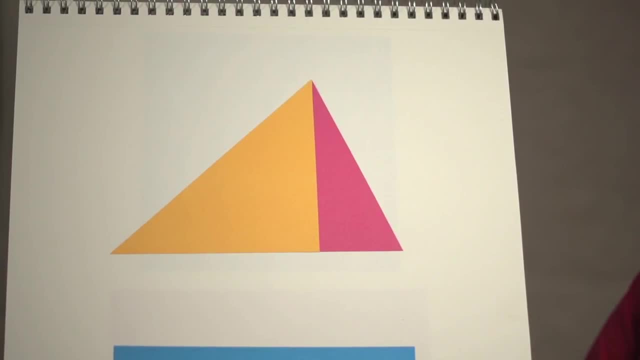 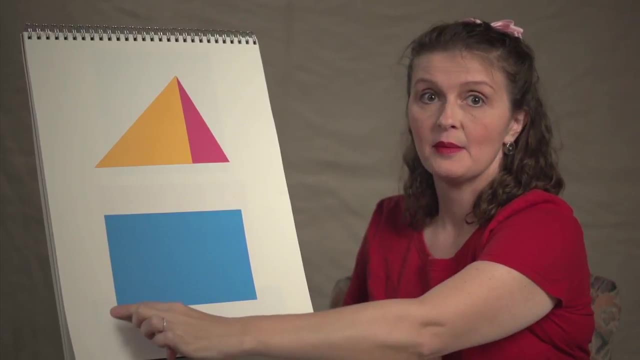 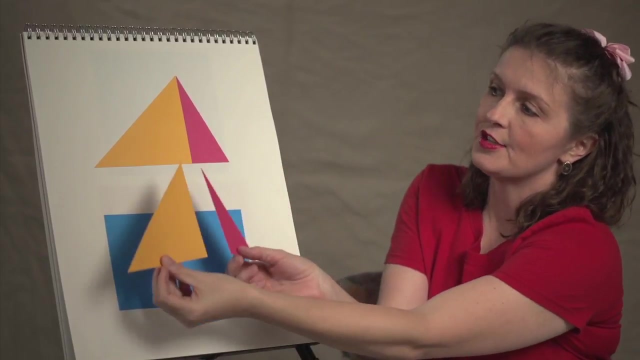 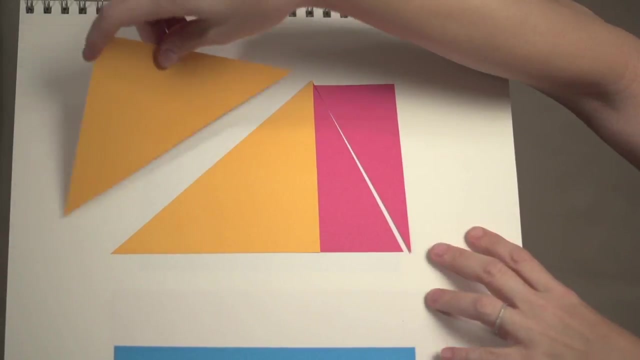 This is actually two triangles put together. Again, if you look at it in its completion, the base is the same as the base here And the height is still the same. If we take an exact copy of this triangle, of these two triangles, and we put them like so, 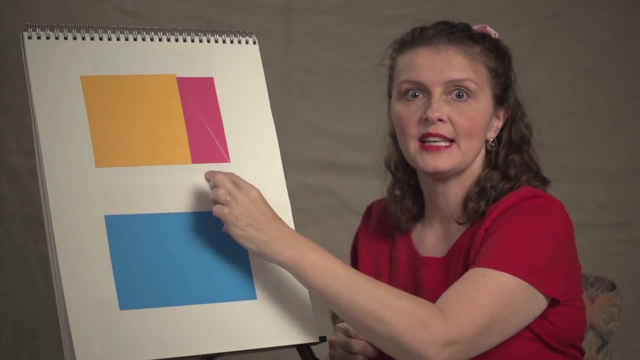 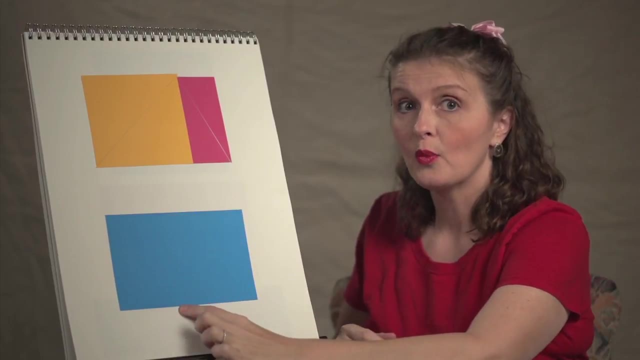 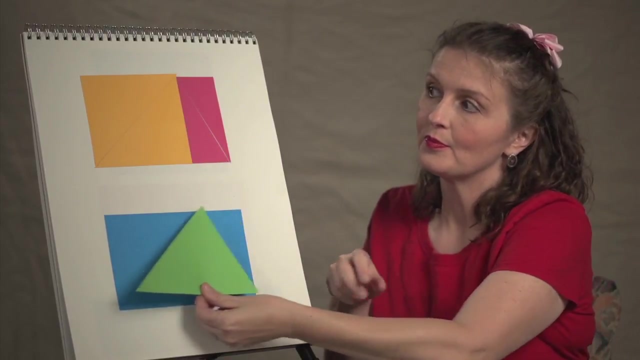 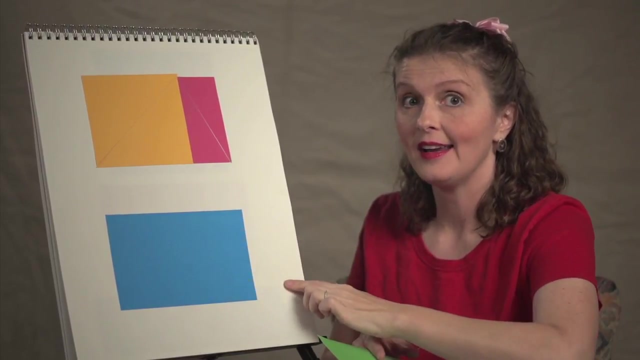 you can see that this makes a rectangle that's the same as this rectangle. So the area, or this part here of the rectangle is really twice the area of the rectangle. So that's how the area of a triangle and rectangle with the same base and height are related.